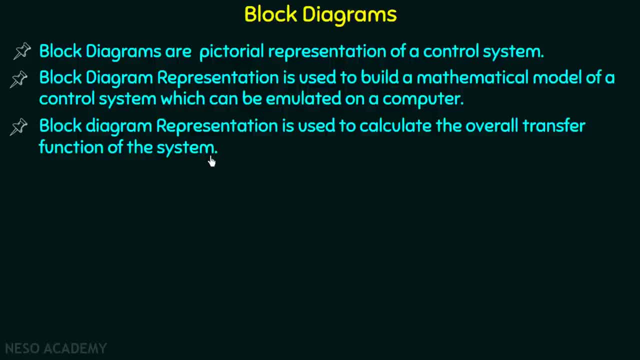 to any given input. we need the transfer function of the system, And block diagram representation helps to find out the overall transfer function of the system. So now we are done with the discussion of introductory points of block diagrams. we will now discuss the elements of a block diagram. 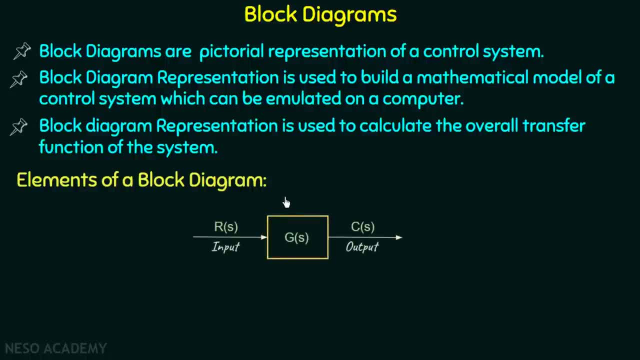 We will start with the basic block diagram representation of a control system that we have already discussed in chapter one, And we all know. this representation consists of a block having two arrows. the arrow or the signal which goes into the block represents the input, the signal which goes out of the block represents the output and the block itself represents the 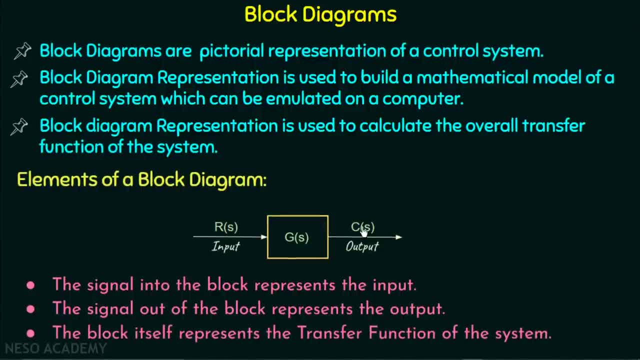 transfer function of the system. But this is the basic block diagram representation of control system. Practically, control systems are more complex in nature. They consist of multiple subsystems. interconnection of many blocks are there which are connected with branches and arrows. So to analyze those complex representations, 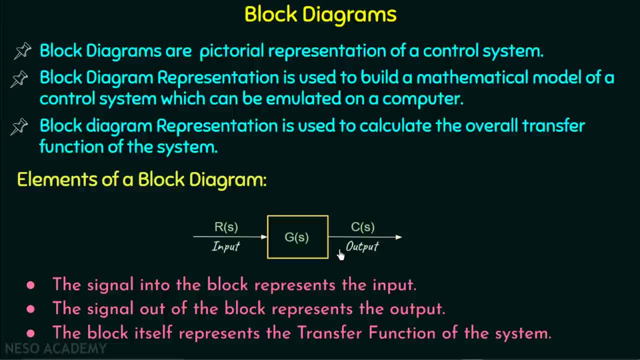 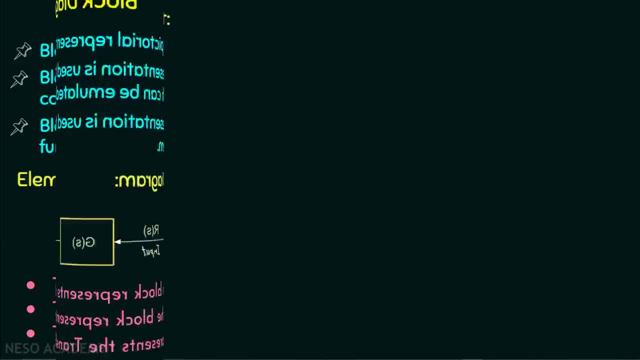 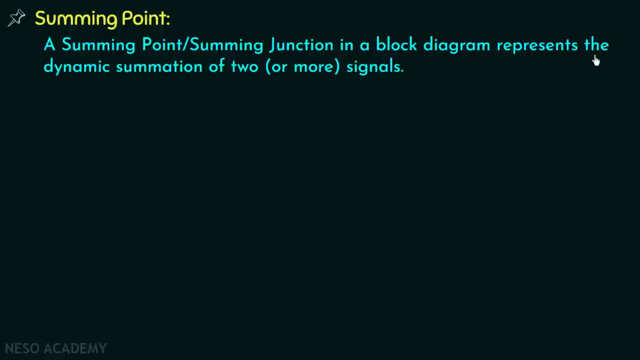 we need to discuss some more elements of block diagrams, like summing point and takeoff point. So now we will move on to the discussion of summing point and takeoff point. We will first see the definition of block diagram representation. A summing point or a summing junction in a block diagram represents the dynamic summation of two or 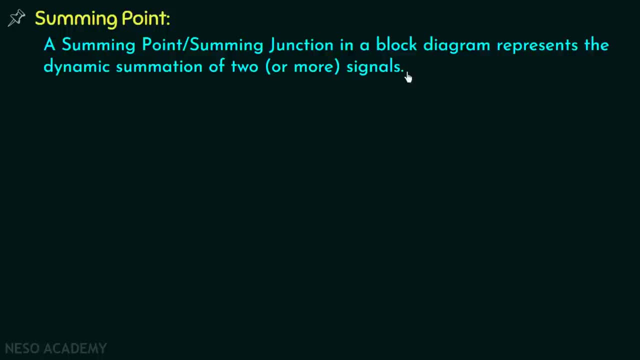 more signals. So wherever we want to add two or more signals in a block diagram, we will use a summing point. This is the symbol of a summing point which is used to add two signals. If this signal is x1 of s and this signal is x2 of s, then the resultant signal will be x1 of s plus x2 of s. 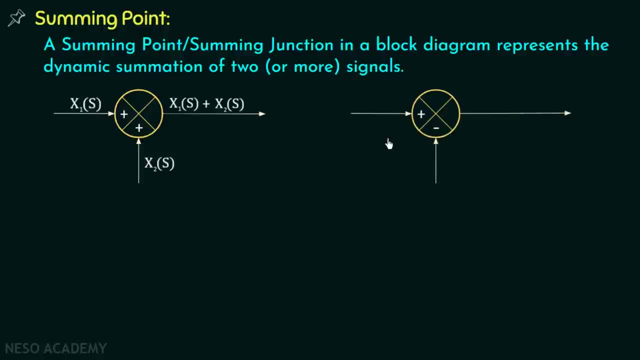 On the other hand, if we want to add two more signals, we will need to add two more signals, And if this is the summing point we are using and this signal is x1 s and this signal is x2 s, then the resultant signal will be x1 s minus of x2 of s. The polarity plays a very important role. 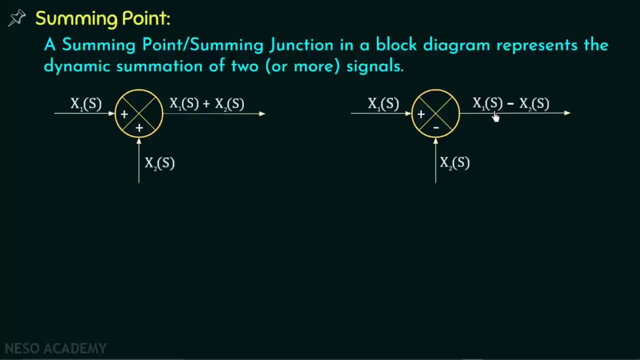 here. If the polarity is positive, then the signal will be positive. If the polarity is negative, then the signal will also be negative. In this case, the polarity of both the signals is positive, and hence the signals are added with a positive sign. 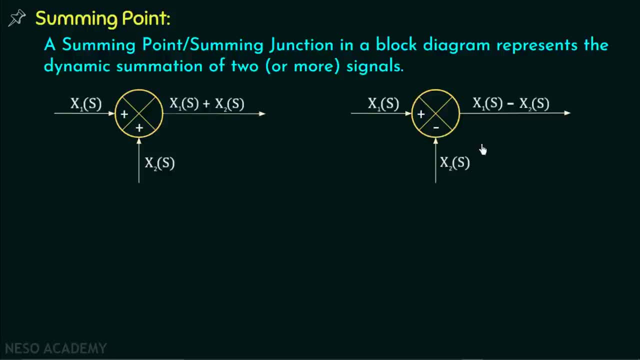 Since we are using the summing point or the summing junction in order to add two or more signals in a block diagram, we can also call this point as adder point. So now we are done with the discussion on summing point. we will now discuss the takeoff point. Takeoff point is also called: 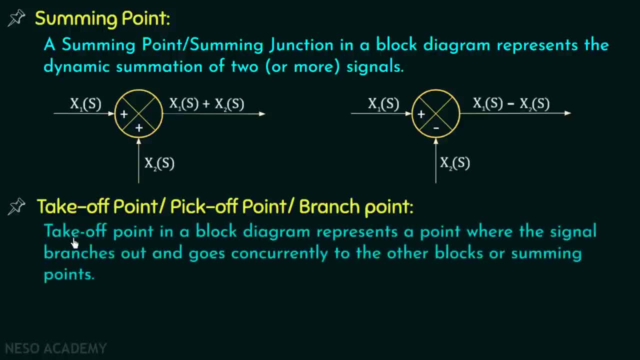 as pickoff point or branch point. So the takeoff point in a block diagram represents a point where the signal is added with a negative sign. So the takeoff point is also called as pickoff point. The signal branches out and goes concurrently to the other blocks or summing points. Or we can say: 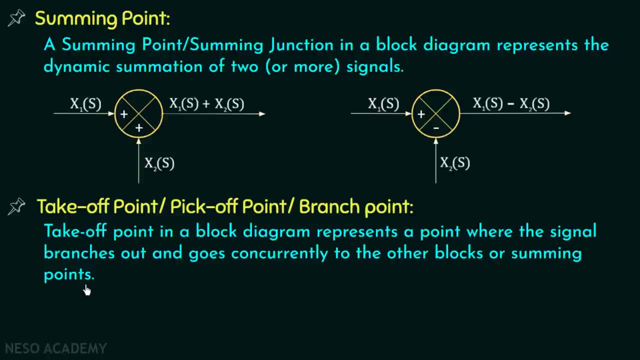 that the takeoff point in a block diagram is a point where the signal distributes to several other branches. Let us understand this with the help of this diagram. This is a branch of a block diagram and we can see that from this point the signal distributes into this branch. So this point. 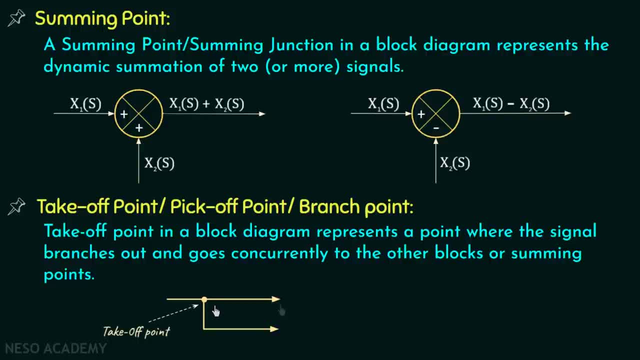 is called as the takeoff point in this block diagram. Similarly, in this block diagram we can see that the signal is added with a negative sign. So this block diagram, this is the takeoff point, as this point distributes this signal into these three. 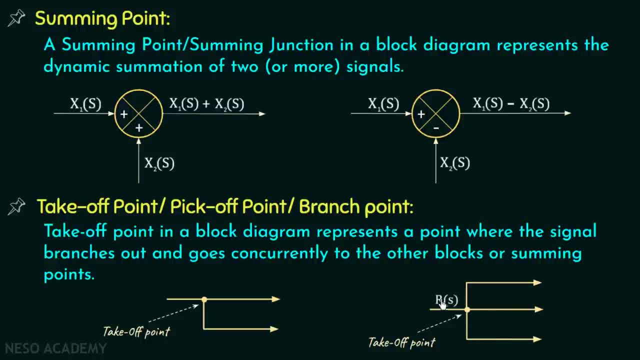 branches. If this signal is R of S, then we can distribute this signal with the help of this takeoff point among these three branches. So this is the basic use of a takeoff point in a block diagram. It distributes the signal from one branch into several other branches. In this way, we are 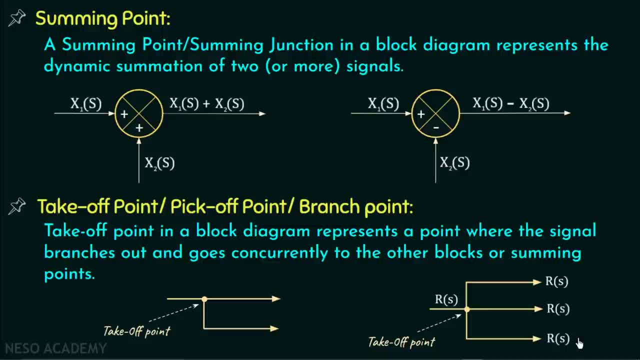 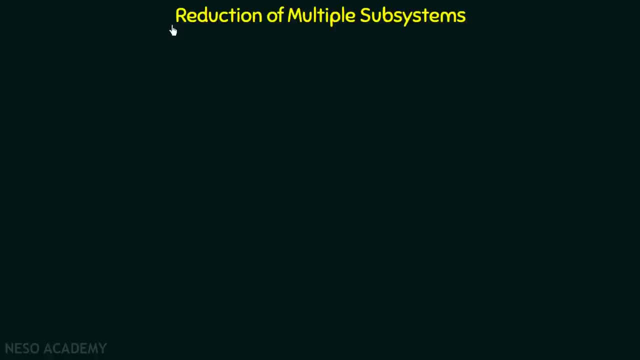 done with the discussion on summing point and takeoff point. We will now move on to the next part. We will move on to reduction of multiple subsystems. As we have already discussed, the practical control systems are complex in nature. They consist of multiple subsystems And, in order, 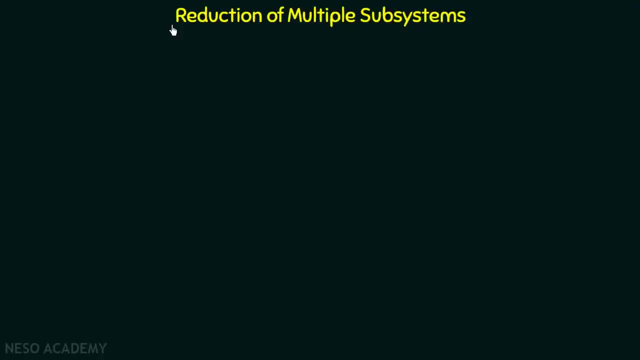 to find out the overall transfer function, we need to reduce those multiple subsystems into a single block. We will discuss this under the topic reduction of multiple subsystems. So, starting with the first point, in order to calculate the output with respect to any given input, we need to 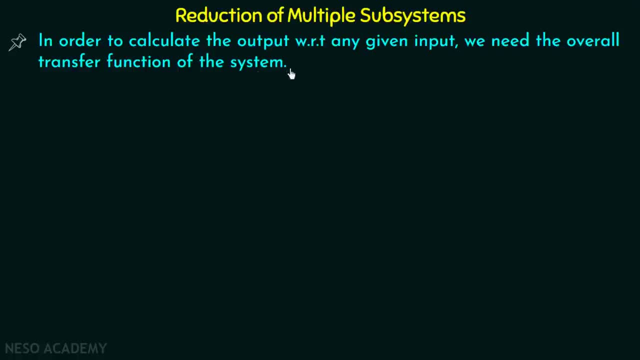 calculate the overall transfer function of the system. We all know this. the transfer function is an important parameter in order to find out the output with respect to any given input. Moving on to the next point, when the system is complex, that is, it is having multiple subsystems, then we need: